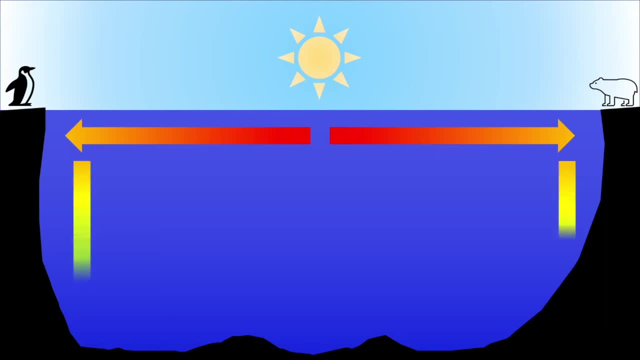 this water will get colder and more dense, making it sink, and when this colder, dense water returns to the equator, it will be subducted underneath the warmer, less dense water, resulting in the creation of water masses. and in the next video I'll talk about the role of salinity in water mass formation. have a great week you.